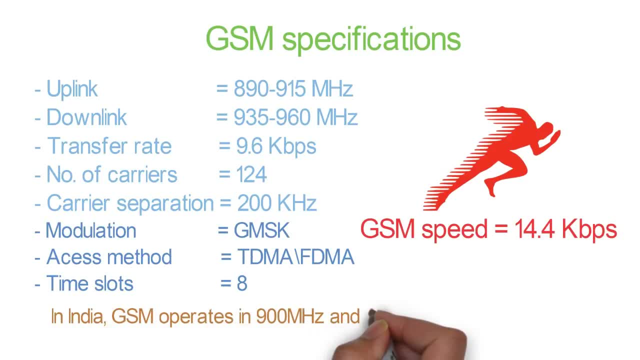 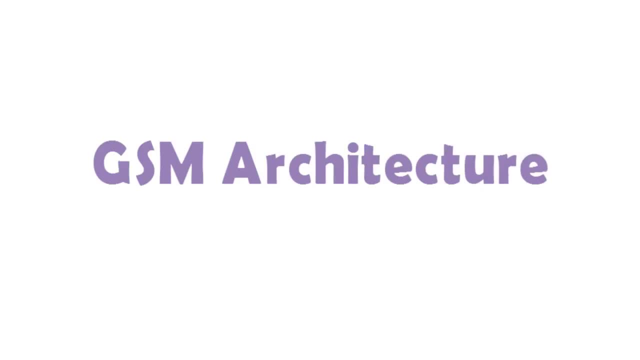 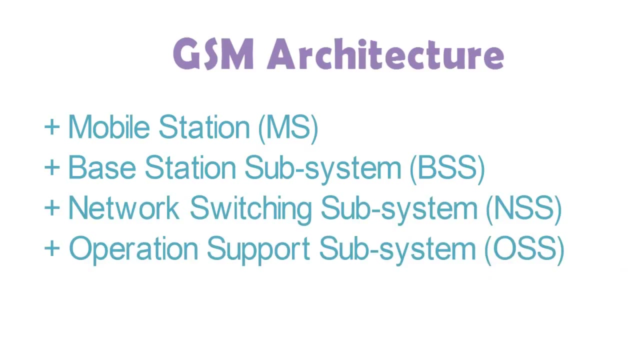 per second. GSM uses different frequency bands in different regions. In India it was 900 MHz and 1,800 MHz. GSM architecture is the basic architecture in a cellular network. It contains four subsystems: Oval station, Base station subsystem, Network switching subsystem, operation support subsystem. 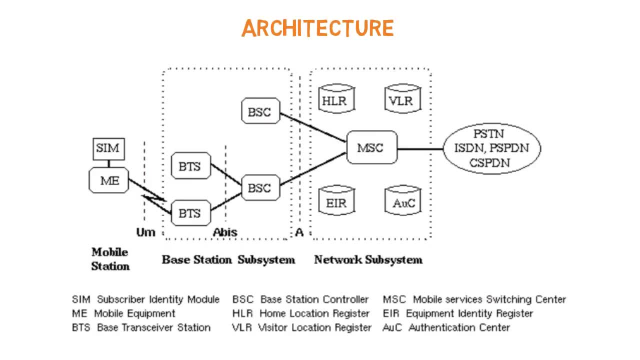 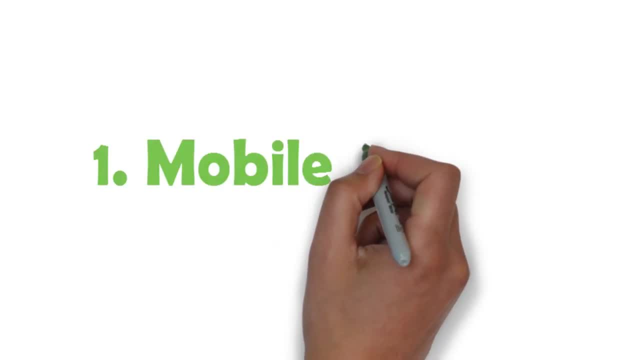 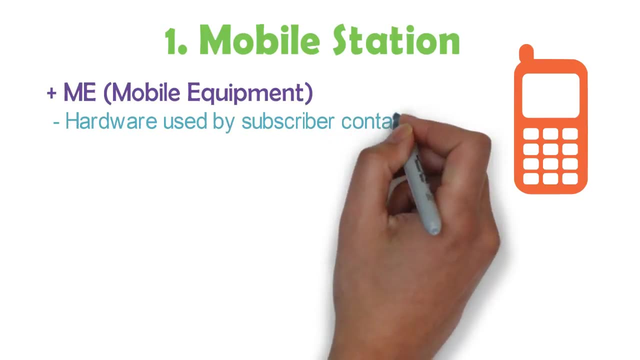 Here it is the representation of each subsystem in the architecture. It is noticed that each subsystem contain some components. let's discuss in detail. first of all is a mobile station. it has two components. mobile equipment: it is the hardware used by a subscriber to access network identified. 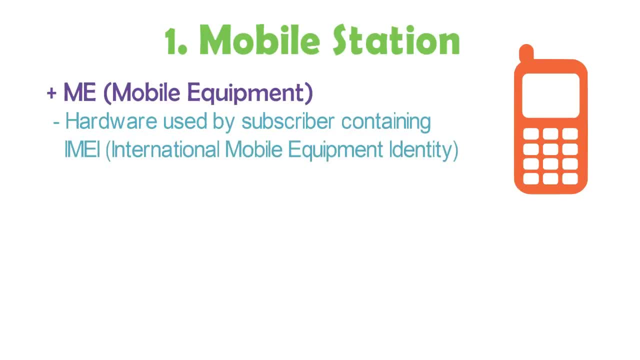 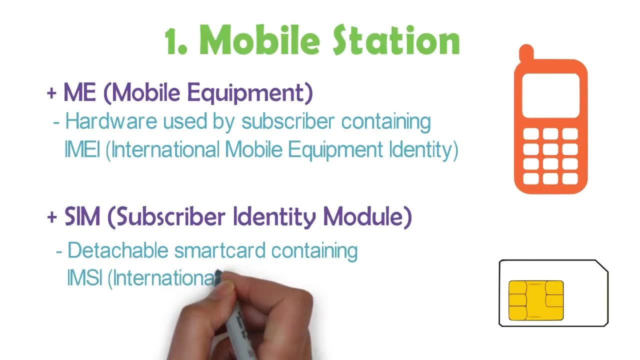 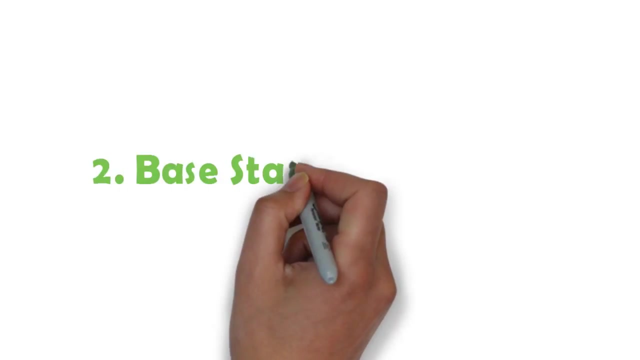 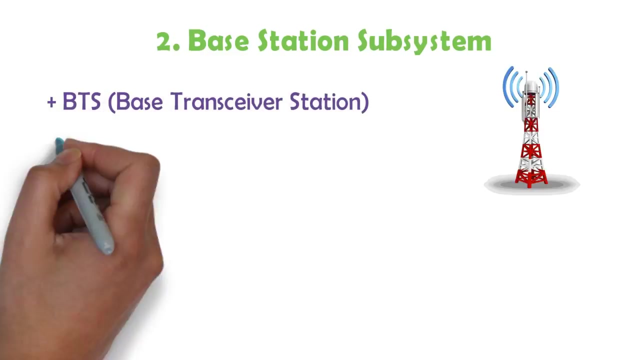 by imei number. international mobile equipment identity. sim subscriber identity module. it is a detachable smart card containing a imsi number: international mobile subscriber identity. it also allows a user to send and receive calls. second subsystem is a base station subsystem. it also contains the two components: a base transceiver system. it is nothing but mobile tower, sir it. 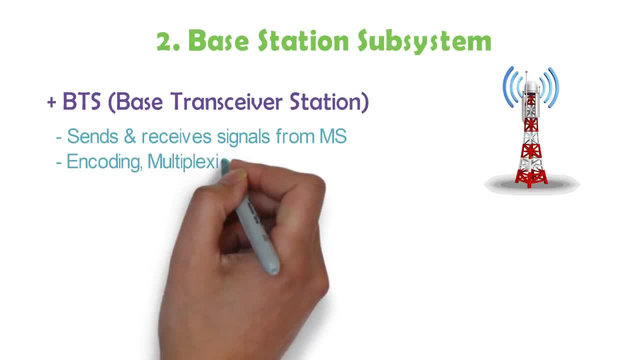 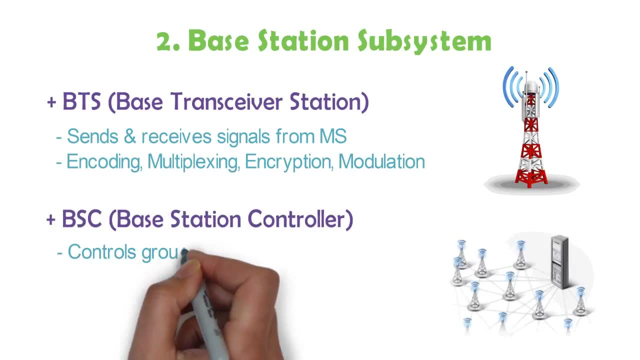 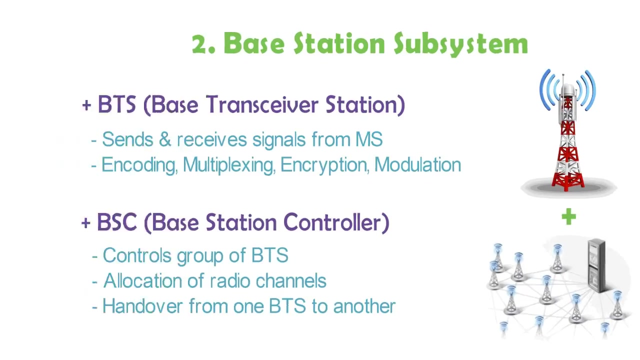 sends and receives signals from mobile phones and performs the various functions like encoding, multiplexing, modulation and encryption. then base stations controller: it controls group of bdss. it allocates radio signals and and over from one bds to another. the third subsystem is a network switching subsystem and it has a five components. the main element is a mobile. 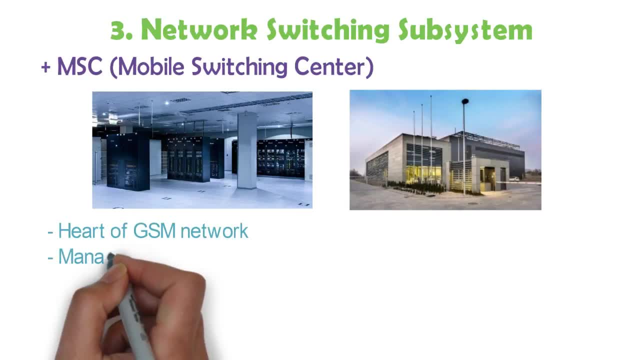 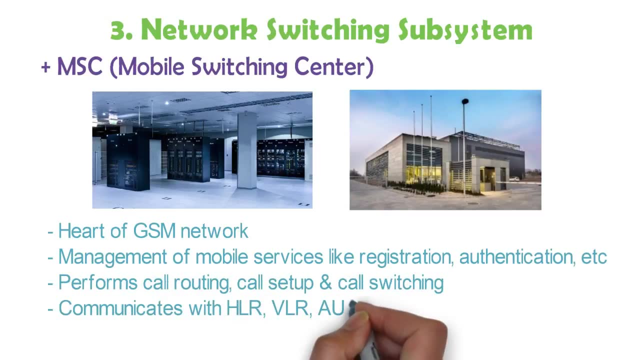 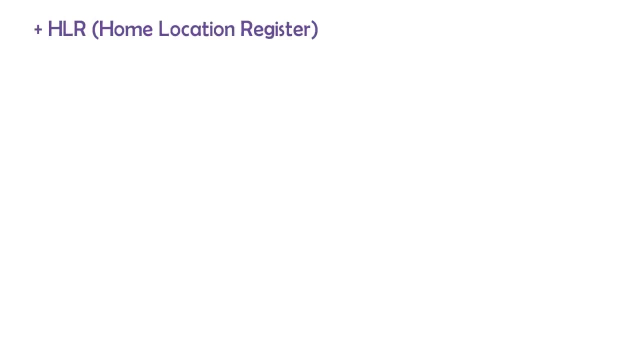 switching center. it is the art of gsm. it manages mobile services like registration, authentication etc. and performs a called routing call setup and the call switching. it communicates with other nss components like hlr, vlr, etc. the second element is a home location register. it is the central. 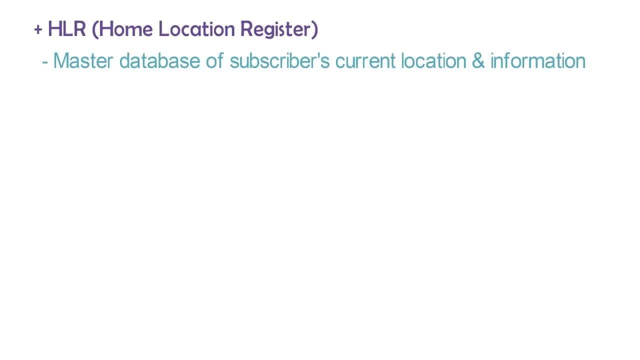 master database of subscribers, imsi, current location and information. third, one is a visitor location register. it is a subset of hlr and also local database of users currently visiting location in other domain. if the user lives in chennai, then it is home network and hlr works here. 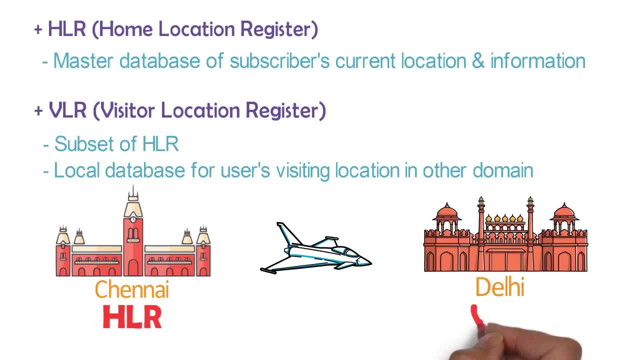 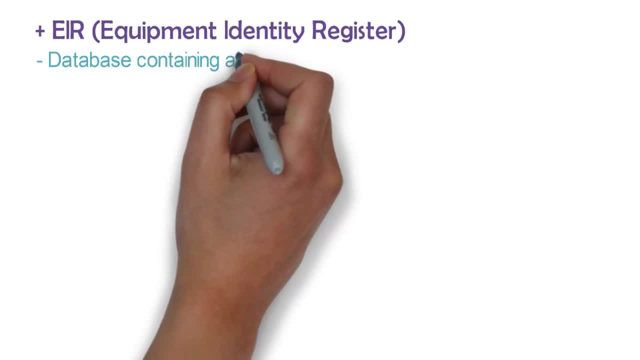 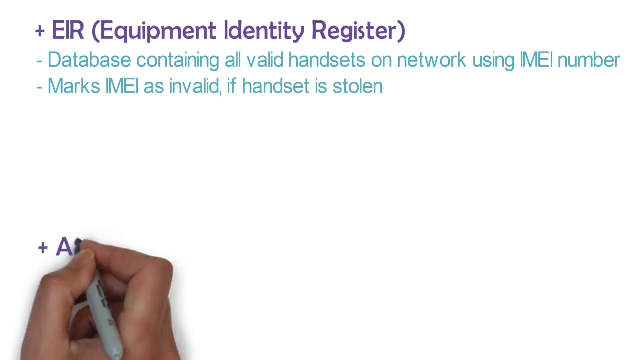 when he travels to delhi, then it is visiting network and vla starts working. the fourth one is a equipment identity register. it is also a database that contains all valid answers on network using ima number. it marks ima as an invalid if an answer is stolen. the element is authentication center, a protected database, and that stores copy of imsa number.